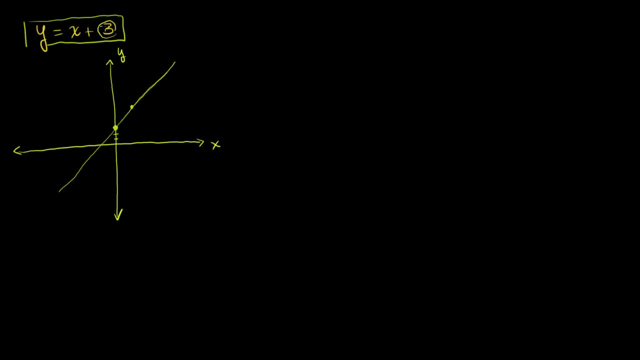 line is a solution to this equation or it represents a pair of x and y that satisfy this equation. So maybe when you take- let's say you take- a x is equal to 5, when x is equal to 5, you go to the line and you're going. 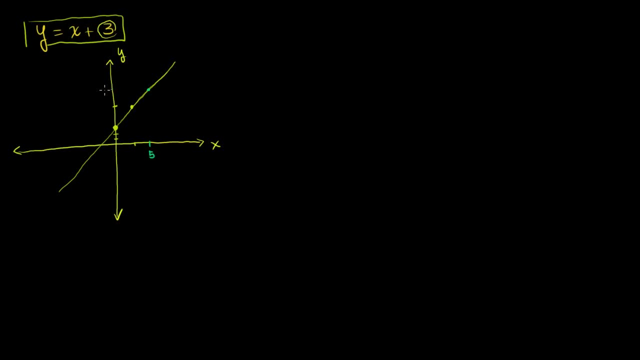 to see gee, when x is equal to 5. on that line, y is equal to 8 is a solution And it's going to sit on the line. So this represents the solution set to this equation. all of the coordinates that satisfy y is equal to x plus 3.. 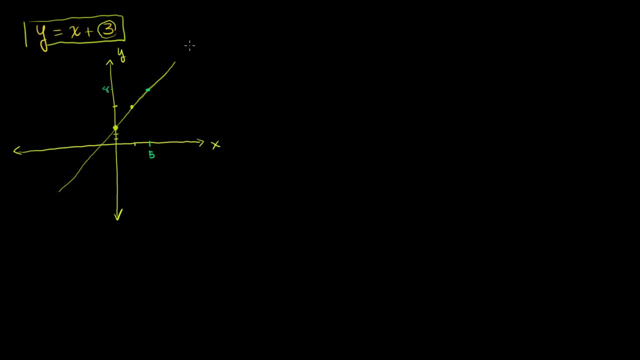 Now let's say we have another equation. Let's say we have an equation. let's say y is equal to negative x plus 3. And we want to graph all of the x and y pairs that satisfy this equation. Well, we could do the same thing. 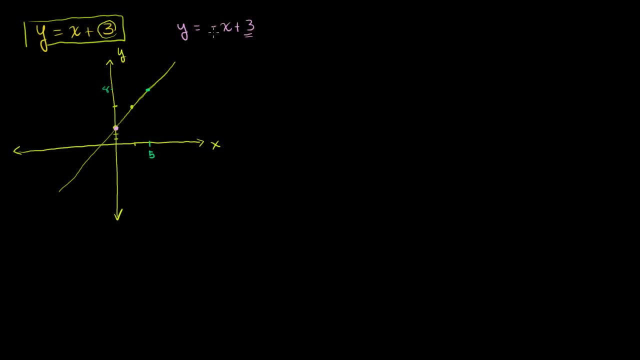 This has a y-intercept also at 3 right there, But its slope is negative 1.. So it's going to look something like this: Every time you move to the right one, you're going to move down one. Or if you move to the right a bunch, you're going to move. 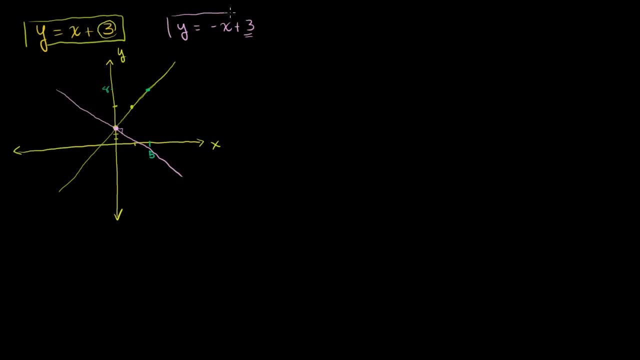 down that same bunch. So that's what this equation will look like. Or every point on this line represents a x and y pair that will satisfy this equation. Now what if I were to ask you: is there an x and y pair that satisfies both? 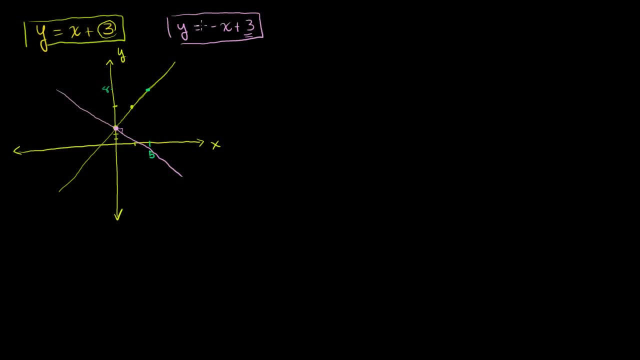 Of these equations. Is there a point or a coordinate that satisfies both equations? Well, think about it. Everything that satisfies this first equation is on this green line, right here, And everything that satisfies this purple equation is on the purple line, right there. 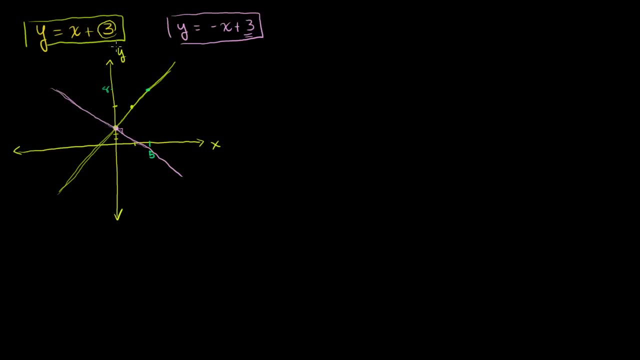 So what satisfies both? Well, if there's a point that's on both lines or essentially a point of intersection of the lines, So in this situation, this point is on both lines And that's actually the y-intercept, the point that's. 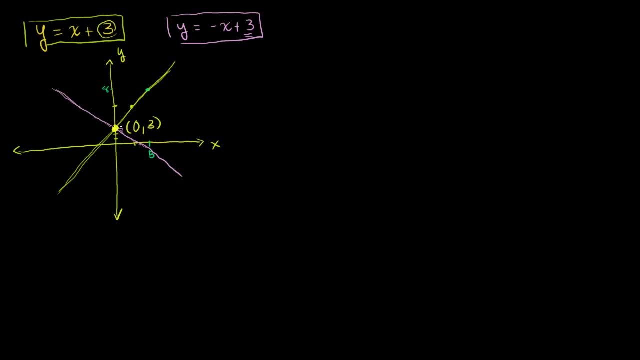 on both lines. 0, 3 is on both of these lines, So that coordinate pair or that x- y pair must satisfy both equations. And you can try it out When x is 0. here 0 plus 3 is equal to 3.. 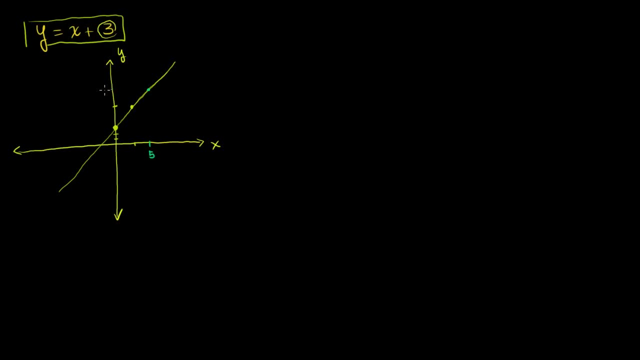 to see gee, when x is equal to 5. on that line, y is equal to 8 is a solution And it's going to sit on the line. So this represents the solution set to this equation. all of the coordinates that satisfy y is equal to x plus 3.. 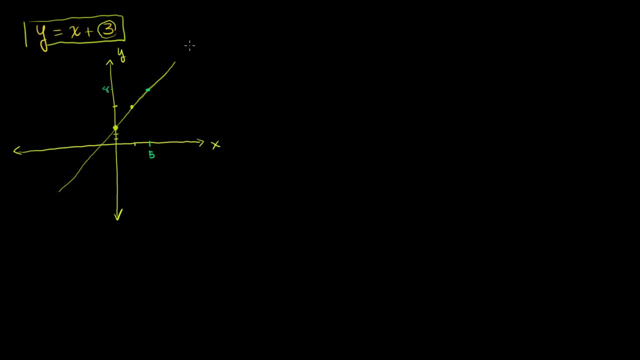 Now let's say we have another equation. Let's say we have an equation. let's say y is equal to negative x plus 3. And we want to graph all of the x and y pairs that satisfy this equation. Well, we could do the same thing. 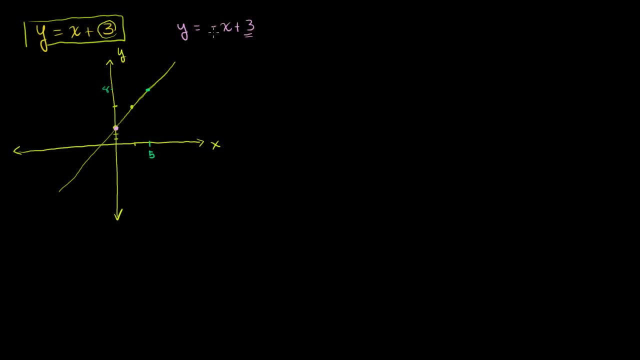 This has a y-intercept also at 3 right there, But its slope is negative 1.. So it's going to look something like this: Every time you move to the right one, you're going to move down one. Or if you move to the right a bunch, you're going to move. 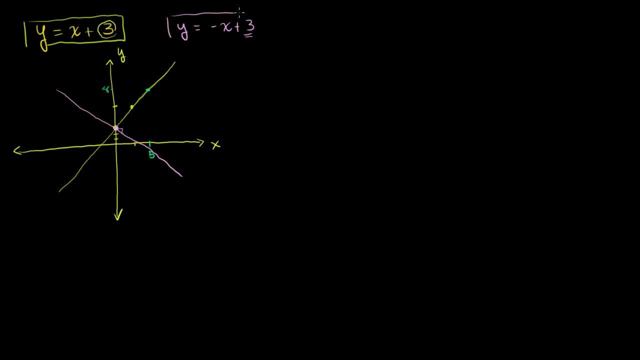 down that same bunch. So that's what this equation will look like. Or every point on this line represents a x and y pair that will satisfy this equation. Now what if I were to ask you: is there an x and y pair that satisfies both? 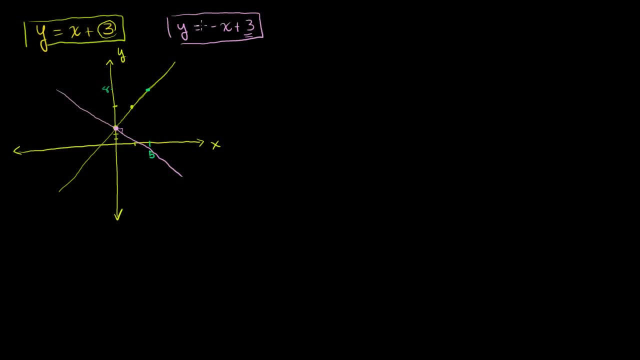 Of these equations. Is there a point or a coordinate that satisfies both equations? Well, think about it. Everything that satisfies this first equation is on this green line, right here, And everything that satisfies this purple equation is on the purple line, right there. 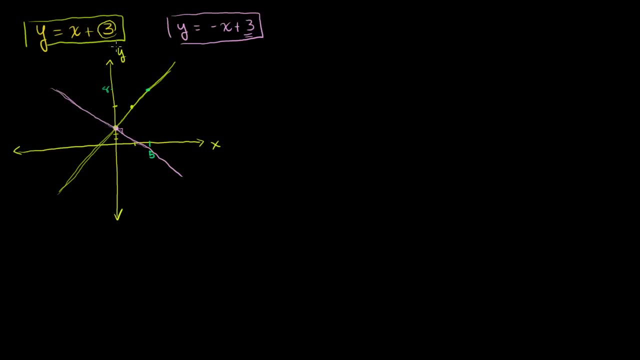 So what satisfies both? Well, if there's a point that's on both lines or essentially a point of intersection of the lines, So in this situation, this point is on both lines And that's actually the y-intercept, the point that's. 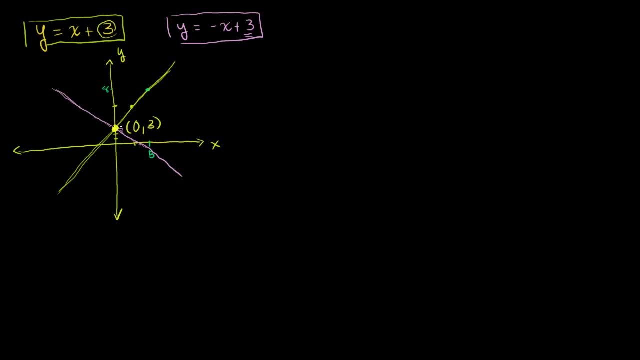 on both lines. 0, 3 is on both of these lines, So that coordinate pair or that x- y pair must satisfy both equations. And you can try it out When x is 0. here 0 plus 3 is equal to 3.. 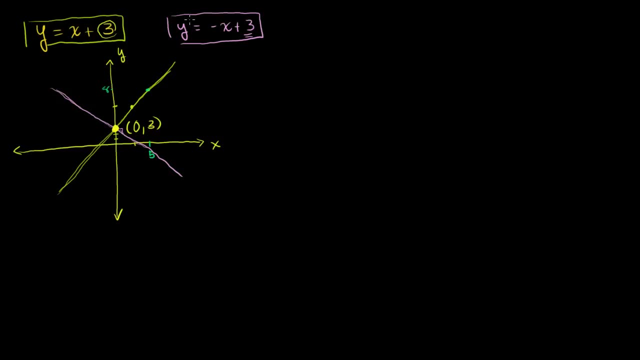 When x is 0, here 0 plus 3 is equal to 3.. It satisfies both of these equations. So what we just did in a graphical way is solve a system of equations. Let me write that down: System of equations. 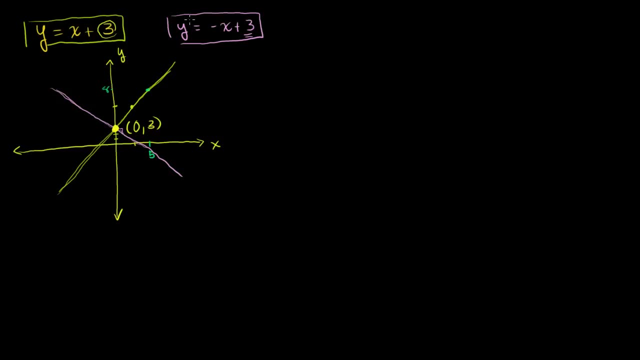 When x is 0, here 0 plus 3 is equal to 3.. It satisfies both of these equations. So what we just did in a graphical way is solve a system of equations. Let me write that down: System of equations. 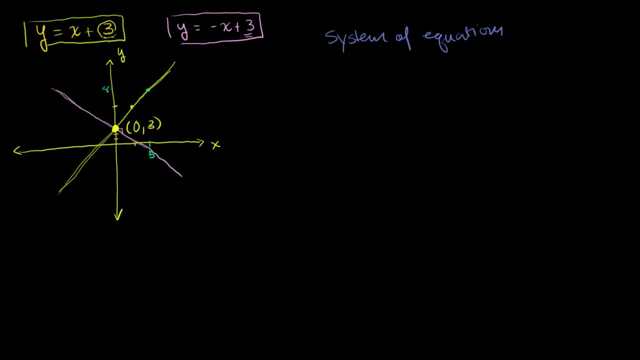 And all that means is we have several equations. Each of them constrain our x's and y's. So in this case, the first one is: y is equal to x plus 3.. And then the second one is: y is equal to negative x plus 3.. 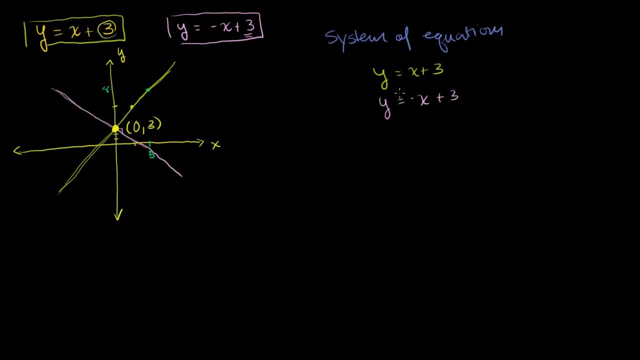 This constrained it to a line in the xy-plane. This constrained our solution set to another line in the xy-plane And if we want to know the x's and y's that satisfy this system of equations, we're going to have to look at the 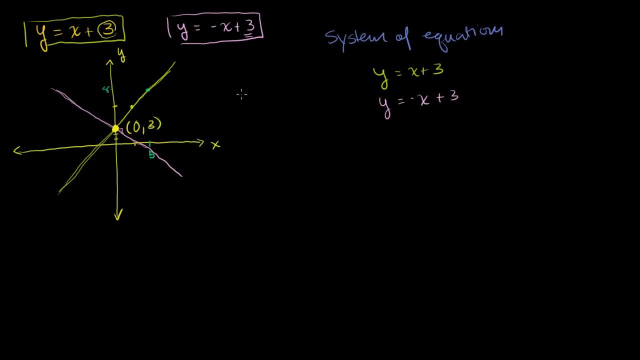 intersection of those lines. So one way to solve these systems of equations is to graph both lines, both equations, and then look at their intersection, And that will be a solution to both of these equations. In the next few videos we're going to see other ways to. 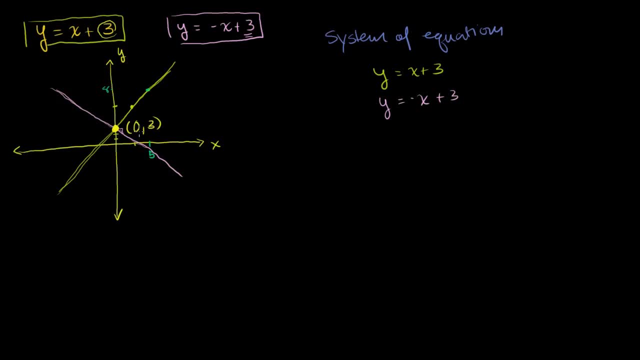 solve it that are maybe more mathematical and less graphical, But I really want you to understand the graphical nature of solving systems of equations. Let's do another one. Another one. Let's say we have y is equal to 3x minus 6.. 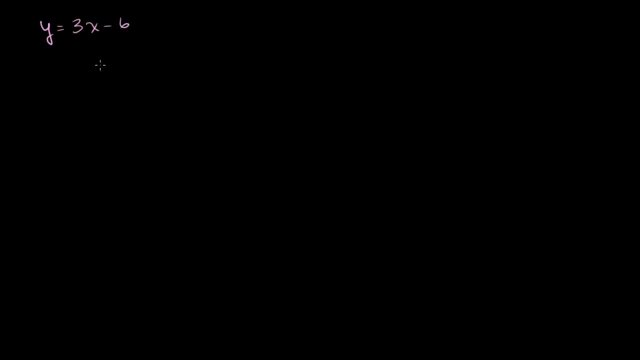 That's one of our equations. And let's say the other equation is: y is equal to negative x plus 6.. And just like the last video, let's graph both of these. I'll try to do it as precisely as I can. 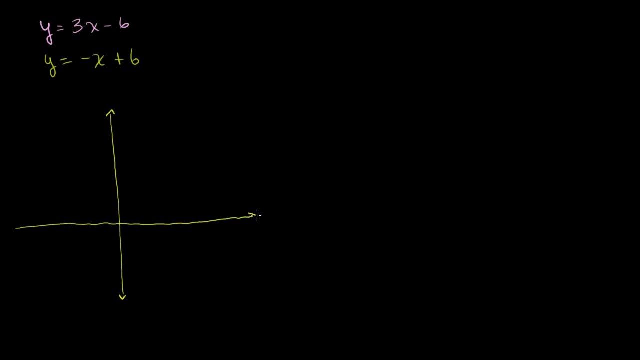 Let's graph both of these. There you go. Let me draw some: 1,, 2,, 3,, 4,, 5,, 6, 7,, 8,, 9, 10.. 1,, 2,, 3,, 4,, 5,, 6,, 7,, 8,, 9,, 10.. 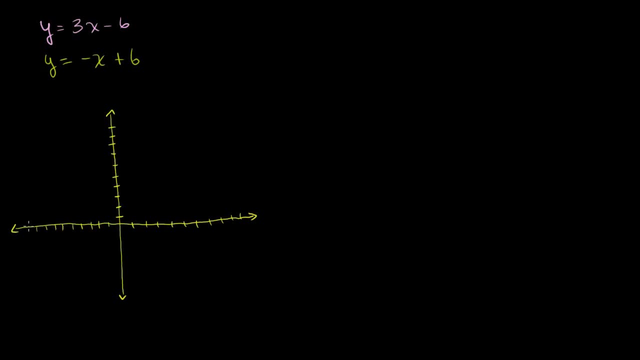 And then 1,, 2,, 3,, 4,, 5,, 6,, 7,, 8,, 9, 10.. I should have just copied and pasted some graph paper here, But I think this will do the job. 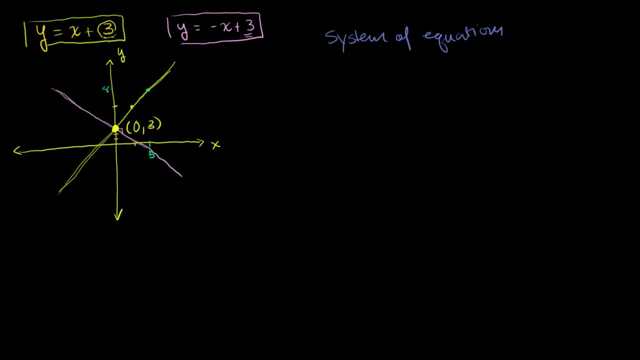 And all that means is we have several equations. Each of them constrain our x's and y's. So in this case, the first one is: y is equal to x plus 3.. And then the second one is: y is equal to negative x plus 3.. 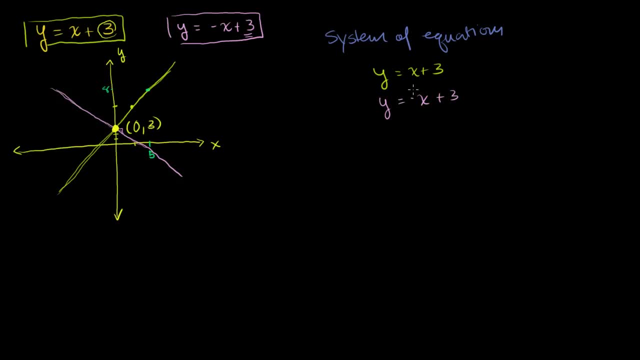 This constrained it to a line in the xy-plane. This constrained our solution set to another line in the xy-plane, And if we want to know the x's and y's that satisfy this system of equations, what we're going to do is we're 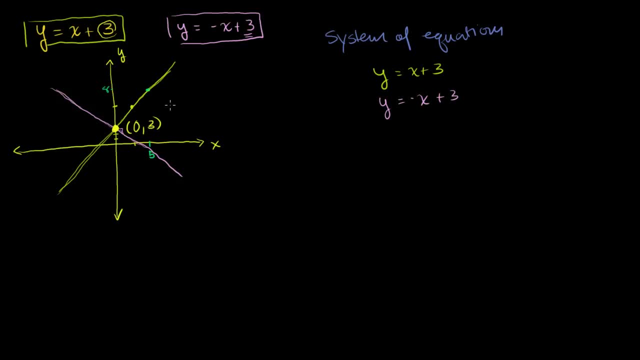 going to solve it by both of these. It's going to be the intersection of those lines. So one way to solve these systems of equations is to graph both lines, both equations, and then look at their intersection, And that will be a solution to both of these equations. 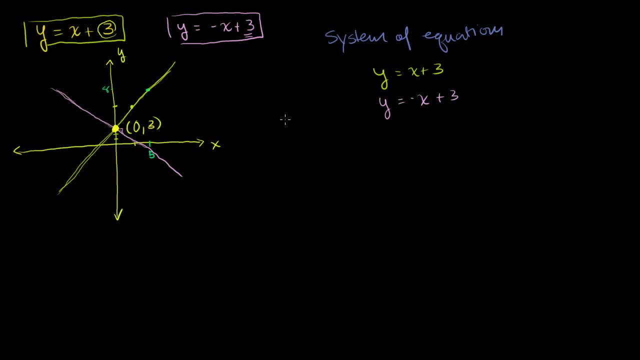 In the next few videos we're going to see other ways to solve it that are maybe more mathematical and less graphical, But I really want you to understand the graphical nature of solving systems of equations. Let's do another one. Let's do another one. 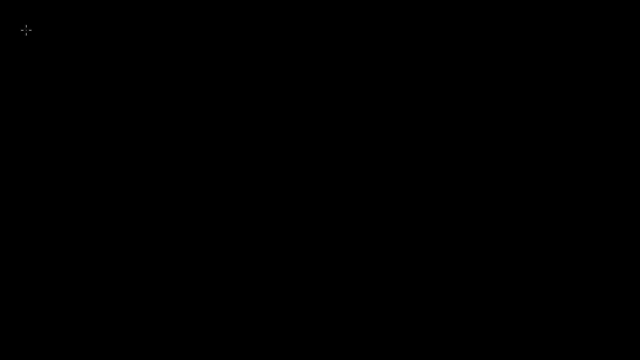 Let's say we have: y is equal to 3x minus 6.. That's one of our equations. And let's say the other equation is: y is equal to negative x plus 6.. And, just like the last video, let's graph both of these. 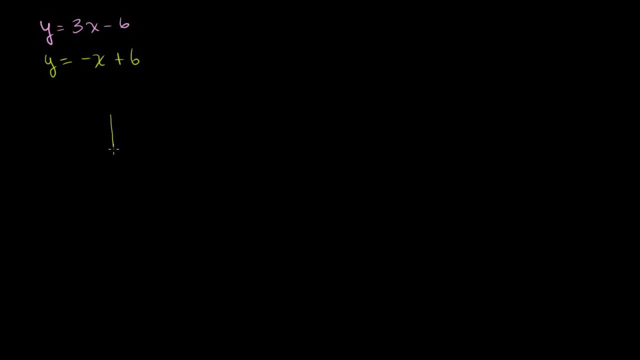 Let's graph both of these. I'll try to do it as precisely as I can. Let's graph both of these. There you go. Let me draw some: 1, 2,, 3,, 4,, 5, 6,, 7,, 8,, 9,, 10.. 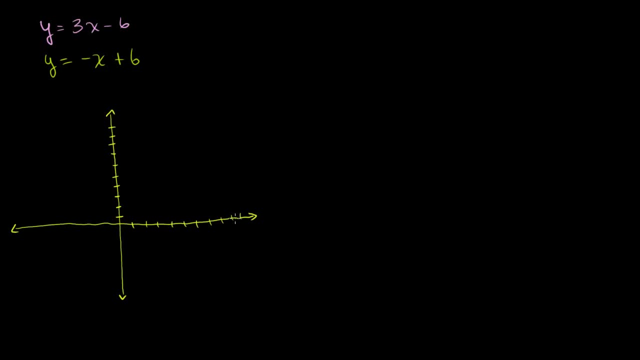 1,, 2,, 3,, 4,, 5,, 6,, 7,, 8,, 9,, 10.. And then 1,, 2,, 3,, 4,, 5,, 6,, 7,, 8,, 9,, 10.. 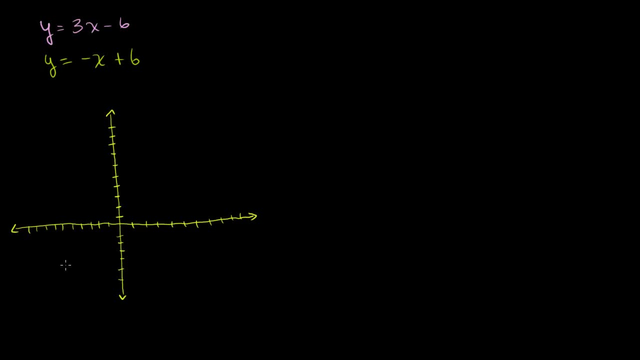 I should have just copied and pasted some graph paper here, but I think this will do the job. So let's graph this purple equation here. Y intercept is negative 6.. So we have 1,, 2,, 3,, 4,, 5, 6.. 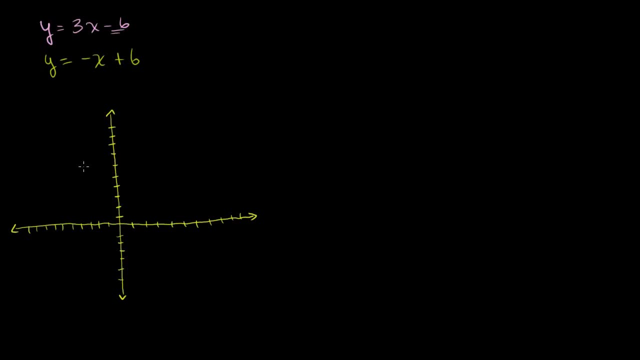 So let's graph this purple equation here: y-intercept is negative 6.. So we have 1.. Let me do another slash: 1,, 2,, 3,, 4,, 5, 6.. So that's y is equal to negative 6.. 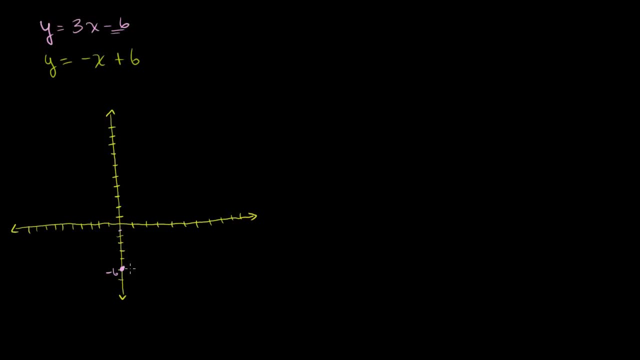 And then the slope is 3.. So every time you move 1,, you go up 3.. You move to the right: 1.. Your run is 1.. Your rise is 1,, 2,, 3.. That's 3, right. 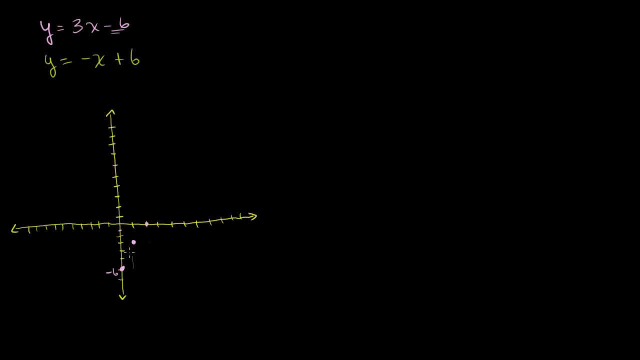 1, 2, 3.. So the equation, the line, will look like this, And it looks like I intersect at the point 2 comma 0, which is right. 3 times 2 is 6 minus 6 is 0.. 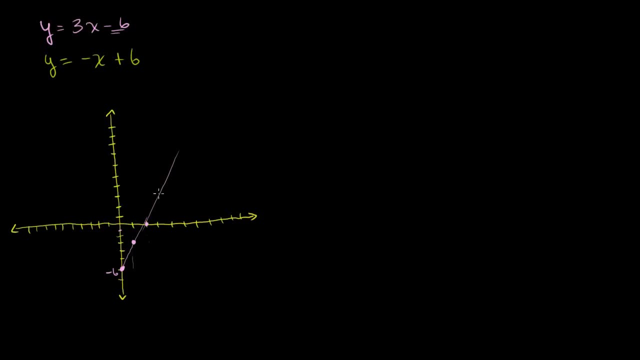 So our line will look something like that. right there, That's that line there. What about this line? Our y-intercept is plus 6.. 1,, 2,, 3,, 4,, 5,, 6.. And our slope is negative 1.. 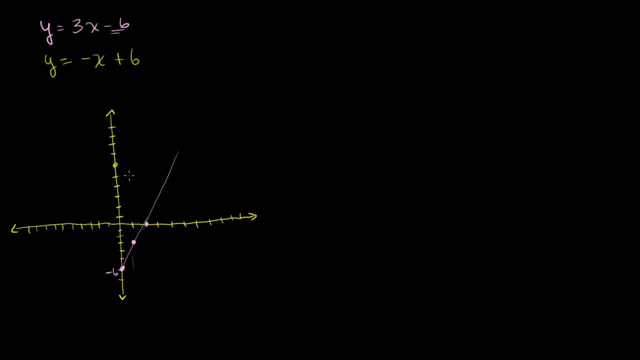 So every time we go 1 to the right, we go down 1.. So you go 1 to the right, you go down 1.. So you go 1 to the right, you go down 1.. And so this will intersect at well when y is equal to 0, x. 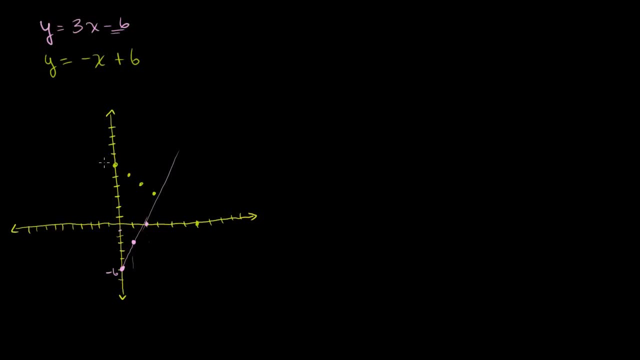 is equal to 6.. 1,, 2,, 3,, 4,, 5,, 6.. So right over there. So this line will look like that the graph. I want to get it as exact as possible, And so we're going to ask ourselves the same question. 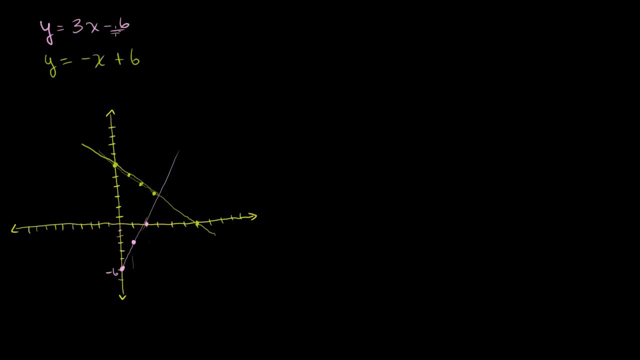 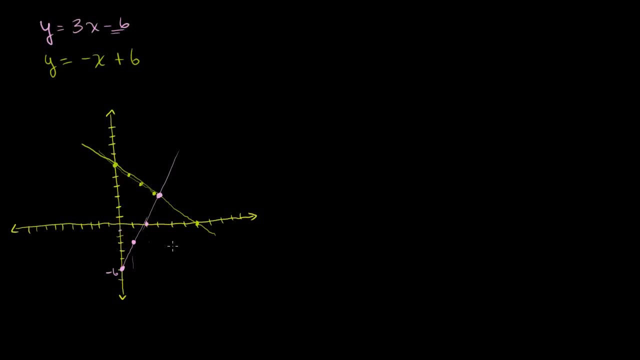 This point lies. This point lies. This point lies on both lines, On both lines there. Let's see if we can figure out what that point is. Just eyeballing the graph here, it looks like we're at 1,, 2,. 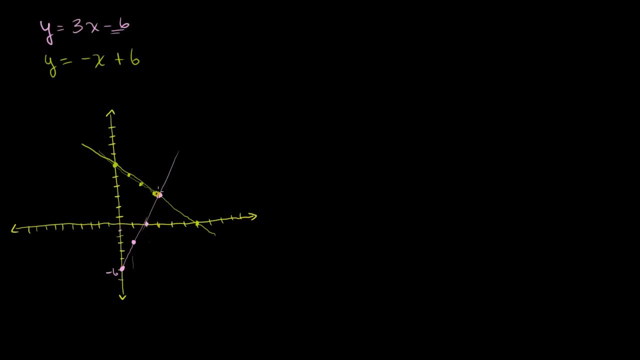 3, comma 1,, 2,, 3.. It looks like this is the same point right there. This is the point 3, comma 3.. I'm doing it just on inspecting my hand-drawn graph, so maybe. 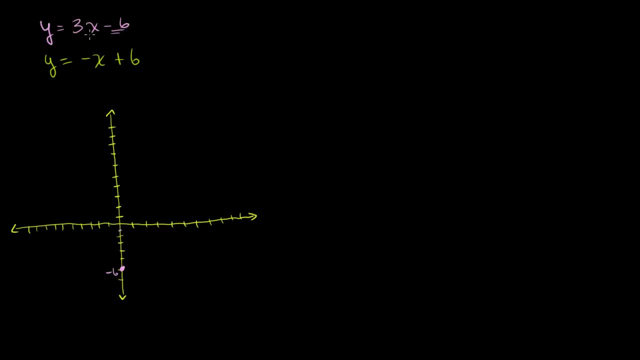 So that's y is equal to negative 6.. And then the slope is 3.. So every time you move 1,, you go up 3.. You move to the right, 1.. Your run is 1.. Your rise is 1,, 2,, 3.. 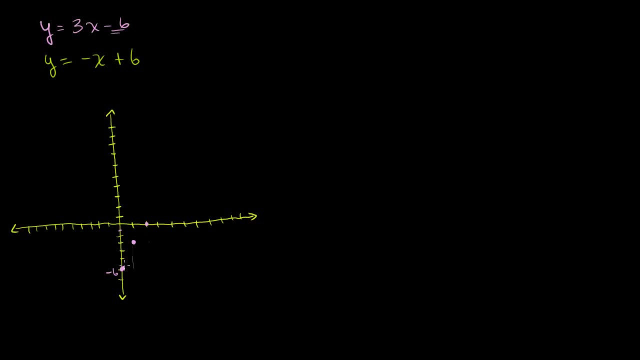 That's 3, right: 1, 2, 3.. So the equation, the line, will look like this, And it looks like I intersect at the point 2, 0, which is right. So 2 is 6.. 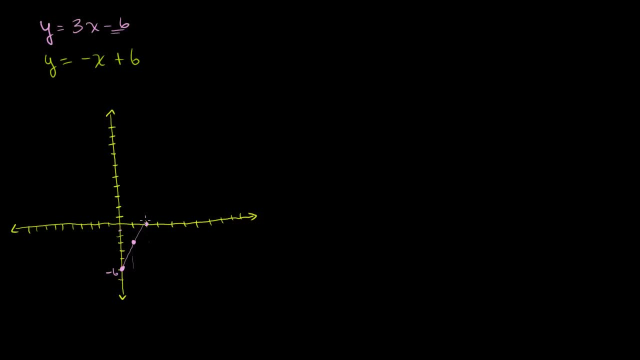 Minus 6 is 0.. So our line will look something like that right there. That's that line there. And what about this line? Our y intercept is plus 6.. 1,, 2,, 3,, 4,, 5,, 6.. 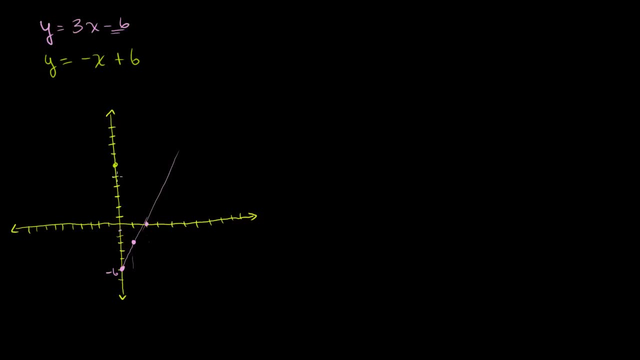 And our slope is negative: 1.. So every time we go 1 to the right, we go down 1.. So you go 1 to the right, you go down 1.. So you go 1 to the right, You go down 1.. 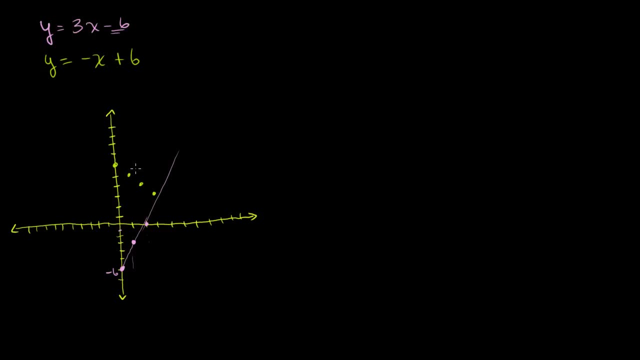 And so this will intersect. This will intersect at well when y is equal to 0,. x is equal to 6.. 1,, 2,, 3,, 4,, 5, 6.. So right over there. 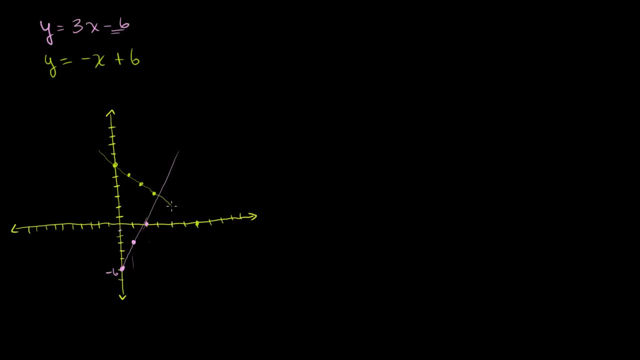 So this line will look like that, the graph. I want to get it as exact as possible, And so we're going to ask ourselves the same question: What is an x-y pair that satisfies both of these equations? Well, you look at it. here it's going to be this point. 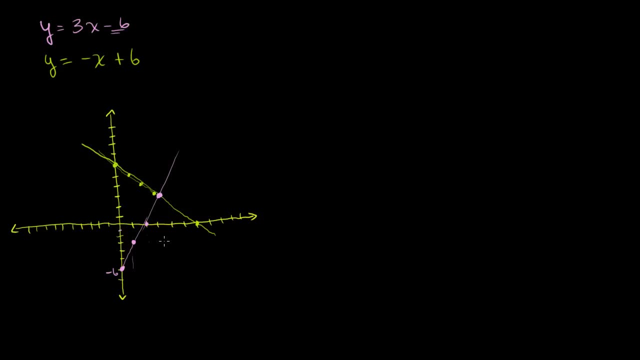 This point lies on both lines, On both lines there. Let's see if we can figure out what that point is. Just eyeballing the graph here, It looks like we're at 1, 2, 3, 1, 2, 3.. 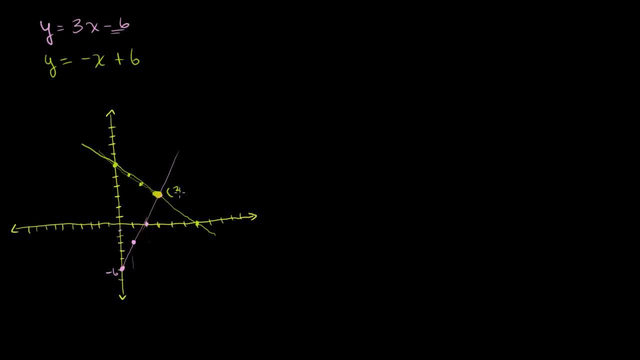 It looks like this is the same point right there, That this is the point 3, 3.. I'm doing it just on inspecting my hand-drawn graph, So maybe it's not the exact. Let's check this answer. Let's see if x is equal to 3, y equals 3..